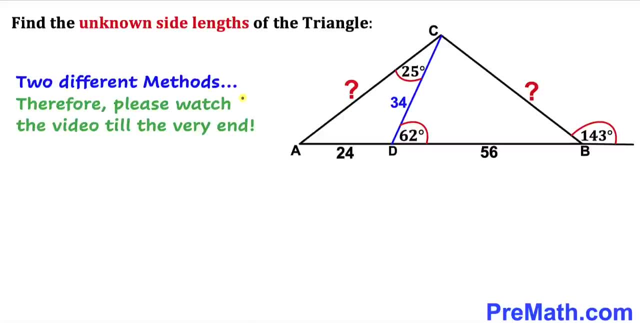 And in this video I am going to share with you two different approaches. So, therefore, please watch the video till the very end. And now let's recall the exterior angle theorem. According to this theorem, the exterior angle of a triangle is equal to the sum of two opposite interior angles, as you can see. 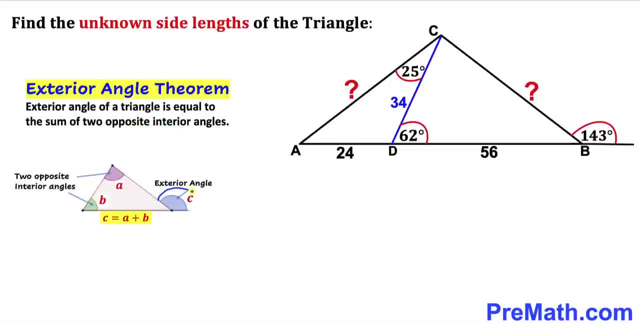 in this diagram. Here we got this C as an exterior angle And A and B are the opposite interior angles, such that this angle C equal to A plus B. So therefore, in our case, this 62 degree angle is our exterior angle and these are our two opposite. 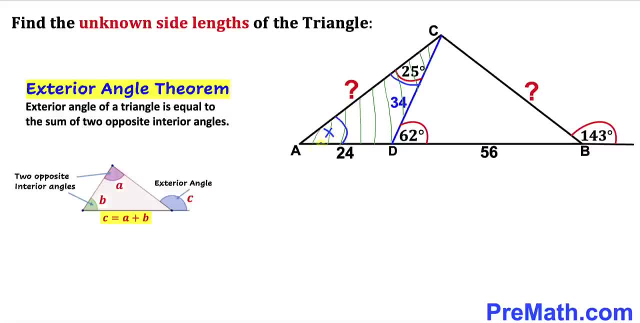 interior angles. Let me go ahead and call this angle X. Then, according to this theorem, we are going to add X plus 25.. Let me write it down: X plus 25 must be equal to 62 degrees. Let's go ahead and subtract 25 degrees from both sides. 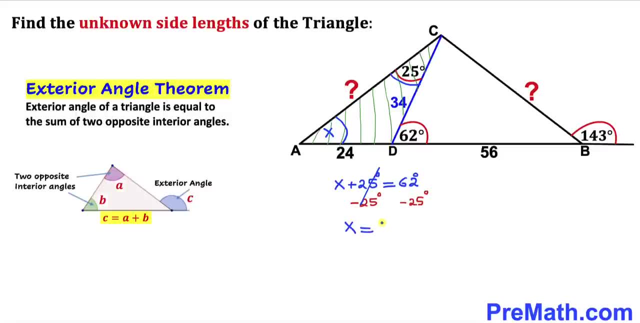 This is gone, So our angle X turns out to be 37 degrees. So, therefore, this angle X is 37 degrees. And now let's focus on this whole straight angle, that's 180 degrees, And we know that this angle is 143 degrees And therefore this angle has got to be 37 degrees. So therefore, we conclude that this 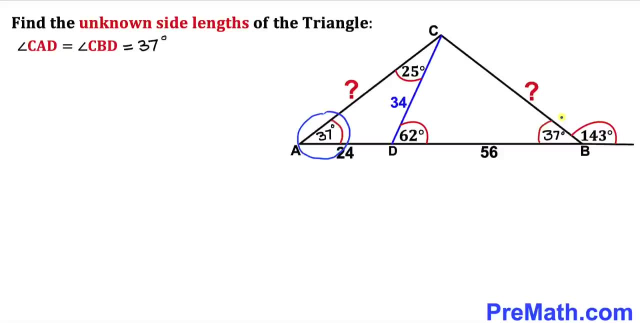 angle CAD and this angle CBD are congruent angles and they are equal to 37 degrees. So therefore we conclude that this triangle ABC is an isosceles triangle and this side length AC congruent to this side length b, c. and since these two sides are congruent, so that means we just need: 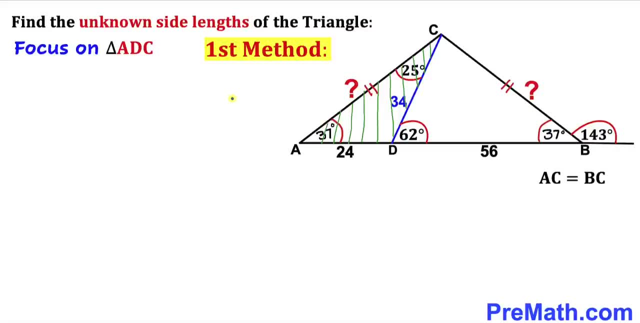 to figure out only one of these sides, and here's our next step. i am going to share with you this very fast method. so, therefore, let's focus on this triangle adc. now let's focus on this straight angle, which is 180 degrees, and we know that this angle is 62 degrees, so therefore, this angle has 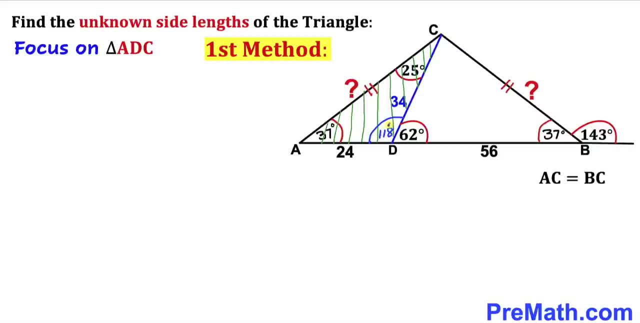 got to be 118 degrees. and now let's recall law of sines: a divided by sine of alpha equals to b divided by sine of beta. let me call this unknown side ac as our side a and the angle opposite to that side of the triangle. adc is going to have to be 180 degrees and we have to figure out. 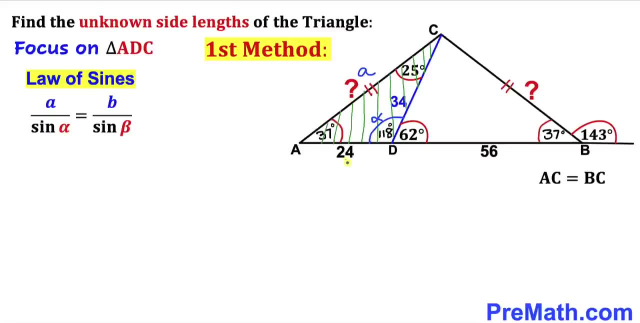 this a is going to be alpha, and let me call this side a, d as side b, and this angle opposite to this side b is going to be angle beta. so let's go ahead and fill in the blanks in this formula, a in our case, we don't know. just leave it there. and now, sine of alpha, in our case, is 118 degrees. 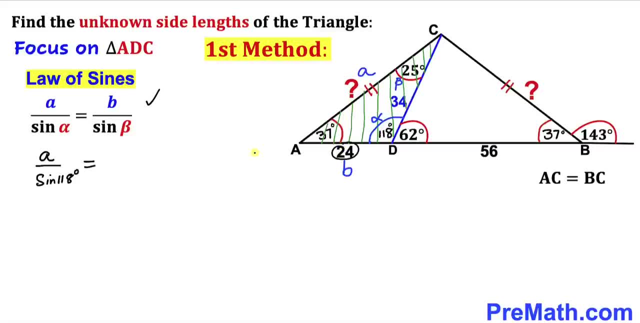 equals to b, in our case is 24, divided by sine of beta is 25 degrees. now let's go ahead and remove this fraction by multiplying sine of 118 degrees on the left hand side and sine of 118 degrees on the right hand side as well. now we can see this sine of. 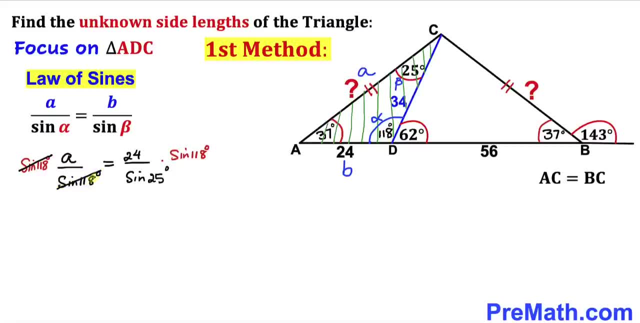 118 degrees on the right hand side as well. now we can see this sine of 118 degrees on the left: 118 degrees, and this sine of 118 degrees is gone. So therefore, A turns out to be equal to 24 times the sine of. 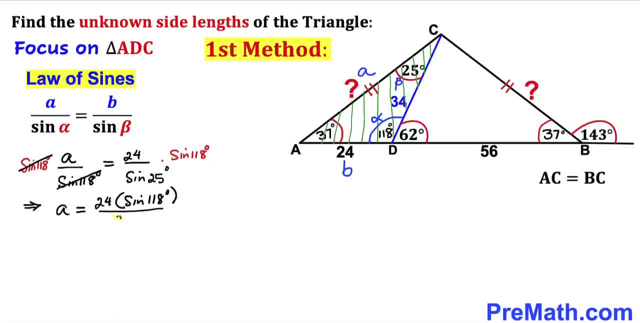 118 degrees divided by sine of 25 degrees, and if we use a calculator, we know that sine of 118 degrees is approximately equal to 0.883, and likewise, a sine of 25 degrees is approximately equal to 0.423.. So let's go ahead and substitute these values over here. So this is going to become: 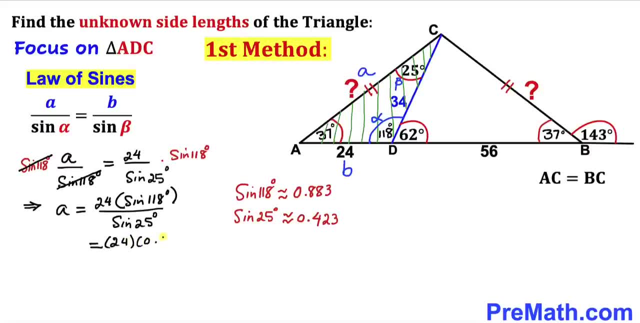 24 times 0.883, all over 0.423. and if we simplify everything on the right hand side, our value turns out to be 50 units. So thus our this AC length turns out to be 50 units, and we know that AC equal to BC. 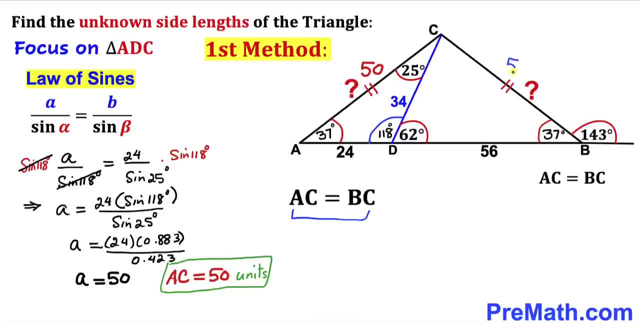 So, therefore, this side length BC is going to be 50 units as well. So that's, our two unknown side lengths turns out to be 50 units, as you can see over here. and now let me go ahead and share with you the second method. 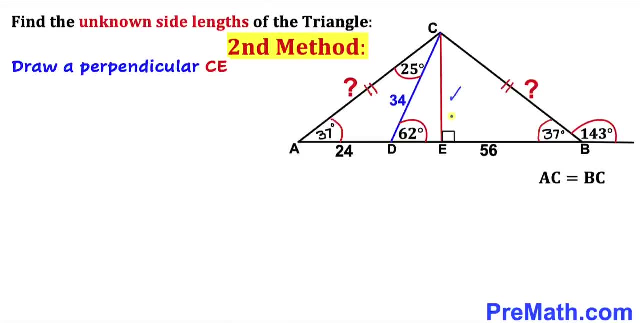 And now let's go ahead and draw a perpendicular CE. as you can see, and we know that this ABC is an isosceles triangle, so therefore this side length AE must be equal to this side length EB, and we know this total length AB is going to be the sum of 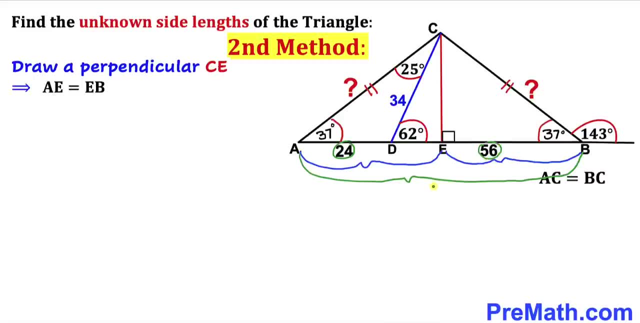 24 plus 56, that is going to give us 80 Units. so therefore, this side length AE is going to be 40 units and likewise, EB is going to be 40 units as well. and now we know that this AD length is 24 units and this AE length is. 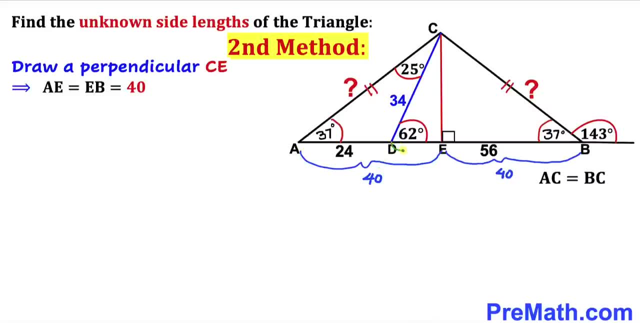 40 units. So therefore this length DE is going to be 40 minus 24 is going to give us 16, so therefore our DE length turns out to be 16. and now let's focus on this triangle DEC, and we know that this is our right triangle. 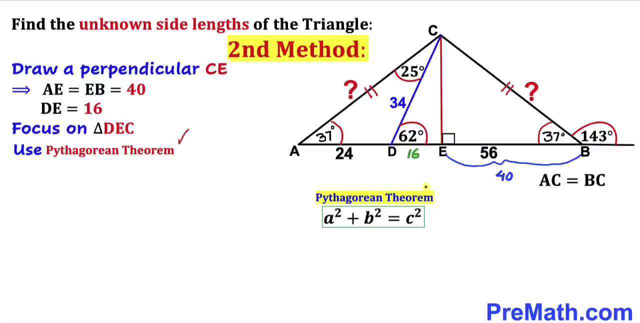 So, therefore, we are going to use the Pythagorean theorem, and here's our Pythagorean theorem: a square plus B square equal to C square. Let me go ahead and call this longest leg as our side C. I'm gonna call this side A and this side B. 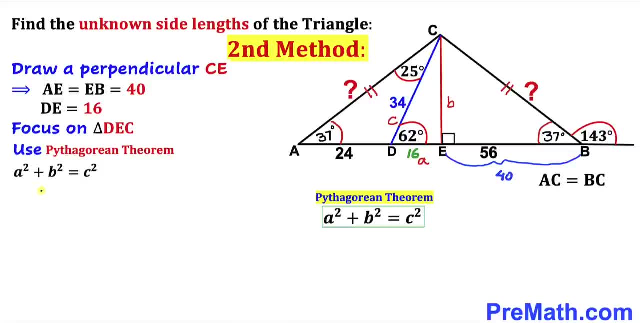 So let's go ahead and fill in the blanks in this Pythagorean formula: A, in our case, is 16, So we are going to write down 16 square and we are going to find the value of B. So let me go ahead and write down B square as it is and C, in our case, is 34, and then the whole. 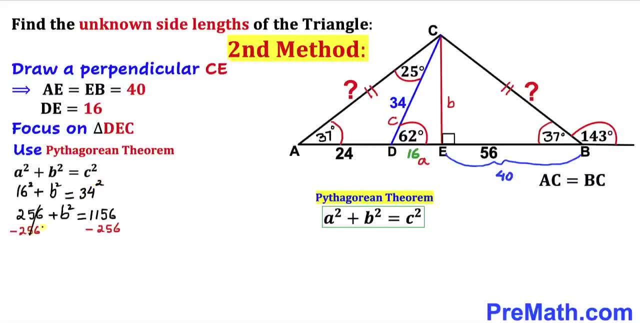 Square. and now let's go ahead and subtract 256 from both sides. This is gone, So B square simply turns out to be 900. let's undo this square by taking the Square root on both side, So therefore our B value turns out to be 30.